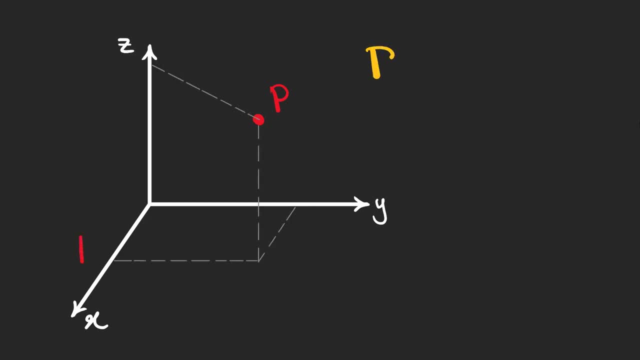 define the point's location relative to them. This point can be specified by three numbers with which we can easily find its location in the 3d space. This is not the only coordinate we can use and we can choose a different coordinate called x prime, y prime and z prime. 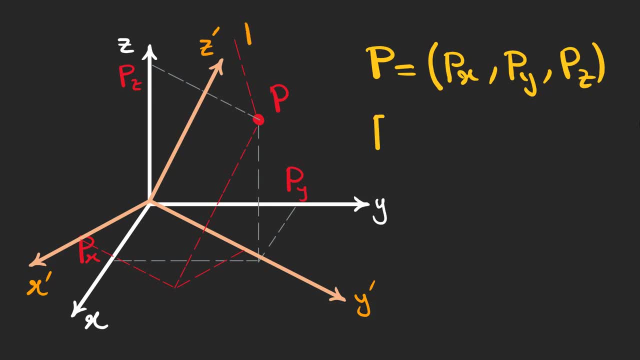 These are the points components on the new frame and three other numbers can be used to show the point in the new coordinates. In this coordinate we can define three unit vectors along each axis and write any vector based on these unit vectors. Now let's consider the same point and let's define three parameters of a spherical coordinate system. 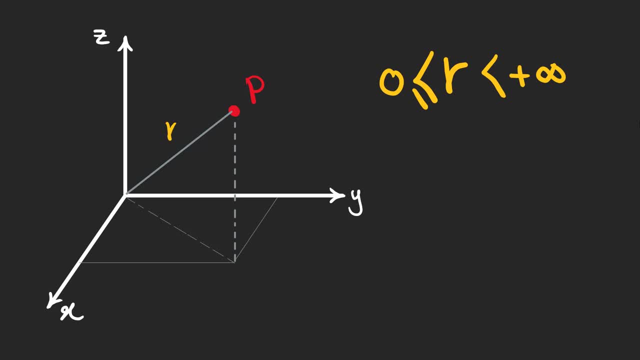 The first parameter is r, which is the distance from the origin to the desired point. The second parameter is phi, and is the angle between the x-axis and the shadow or image of r on the xy plane. And finally, theta is the angle of the z-axis with the line connecting. 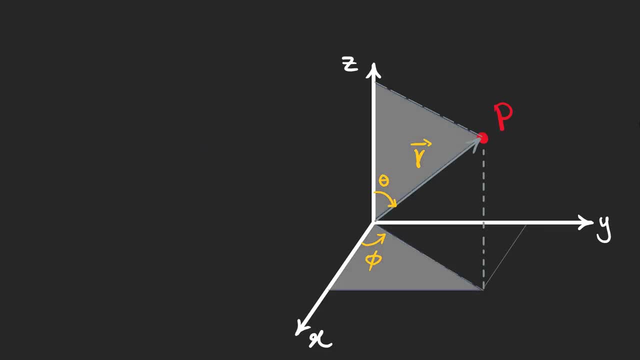 the origin to the point P. Consider these two right triangles and let's write the angle of the z-axis with the line connecting the origin to the point P. Let's write x, y and z based on our new parameters r, phi and theta, using Pythagoras' theorem. 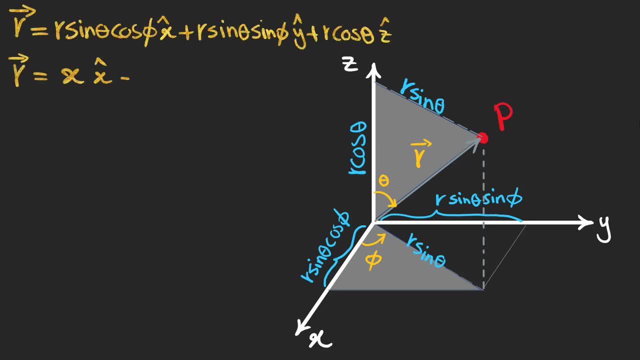 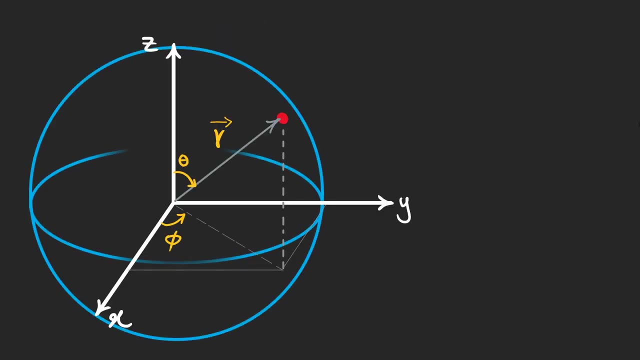 Pay attention that the vector r can be written in these two forms using Cartesian unit vectors. But the question here is how we can use these expressions to drive the unit vectors r hat, phi hat and theta hat in a spherical coordinate. Suppose that the point lives on the surface of a sphere with radius r. Consider the plane tan. 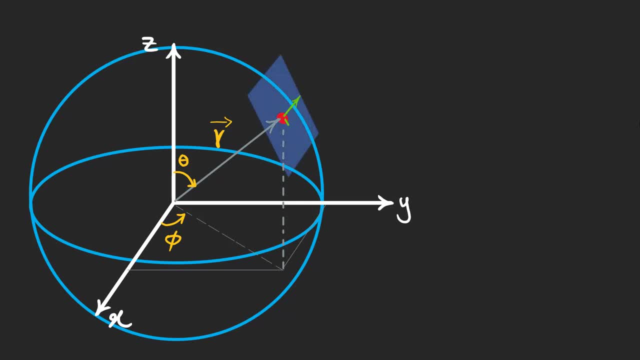 tangential to the surface of the sphere. at this point, Phi hat and theta hat are two unit vectors living on this plane, and r hat is perpendicular to the plane and therefore to phi hat and theta hat. To find these unit vectors we can take the partial derivative of r with respect to each. 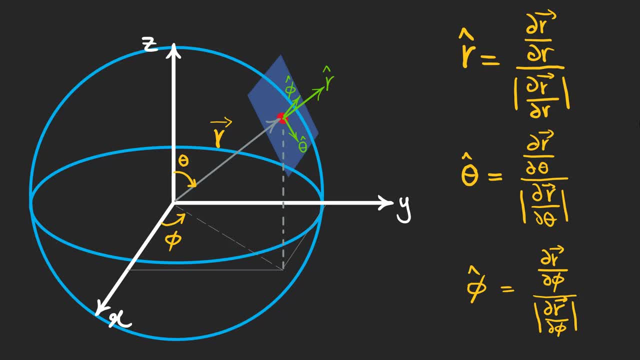 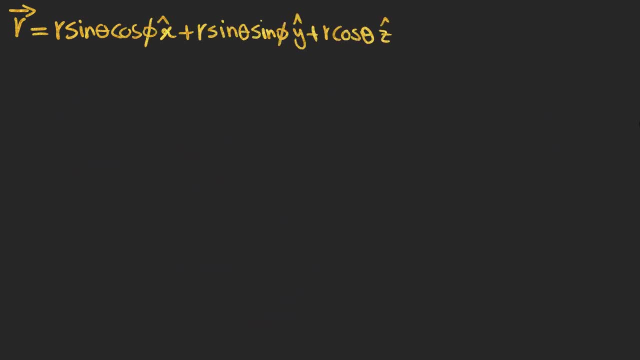 component. to find how r changes in this direction and divide it by its magnitude. to find the unit vectors. We already know r in terms of these three spherical coordinates. To find r, first take the partial derivative of the vector r with respect to r, Then find its magnitude by: